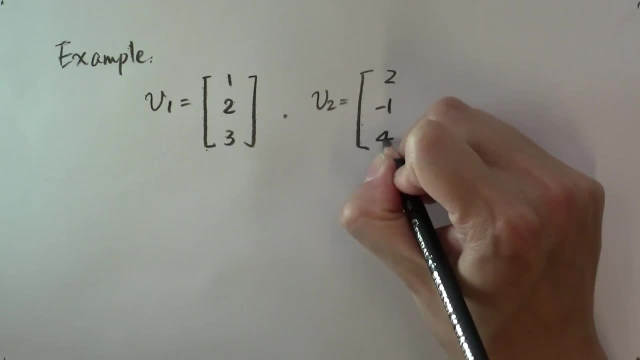 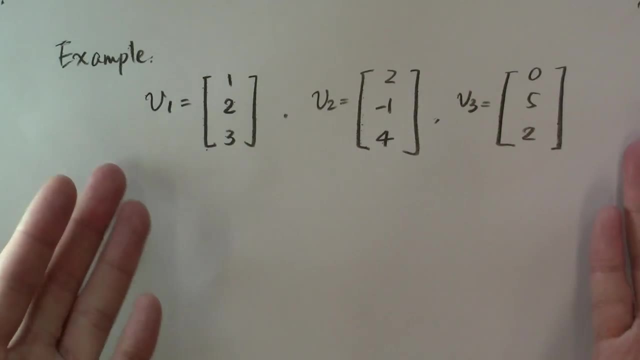 is 2, negative 1, 4.. And v sub 3 is 0,, 5, 2.. Let me ask you: are these three vectors linearly independent or not? How do we go about finding the answer to that question? Well, we begin with the definition. 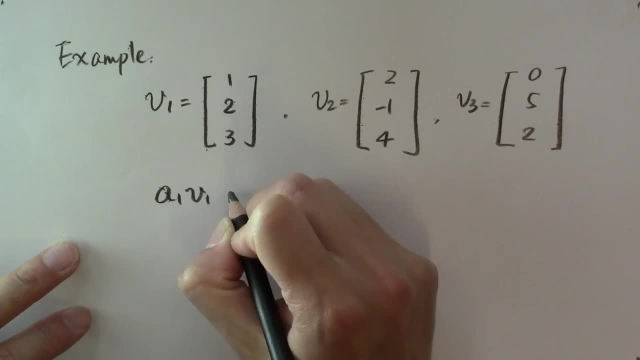 Let's look at the equation: a sub 1 times v. sub 1 plus a sub 2 times v. sub 2 plus a sub 3 times v sub 3, equal to the zero vector If there is a set of numbers, a sub 1, a. 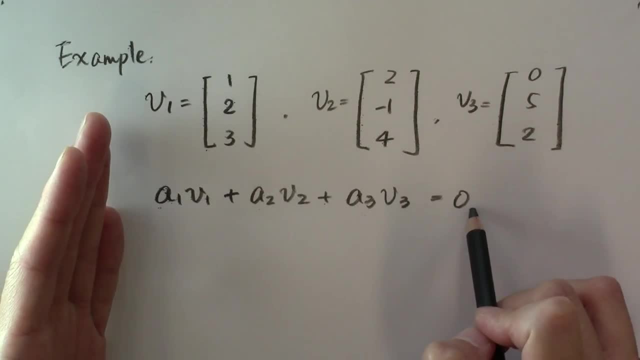 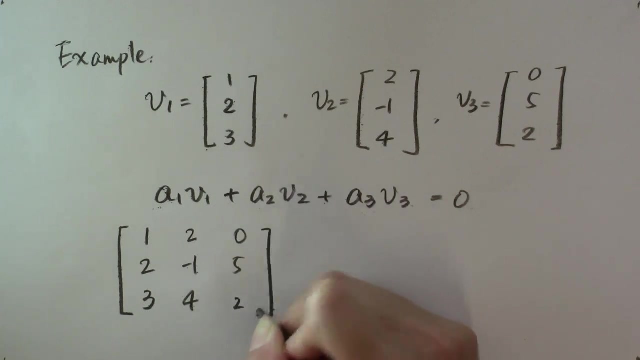 a sub 2, a sub 3, that satisfy this equation and they're not all zeros, then this set of vectors is not linearly independent. Otherwise it will be linearly independent And we recognize that the left-hand side is exactly the equation: 1, 2, 3, 2, negative, 1, 4, 0,, 5, 2, multiplying the. 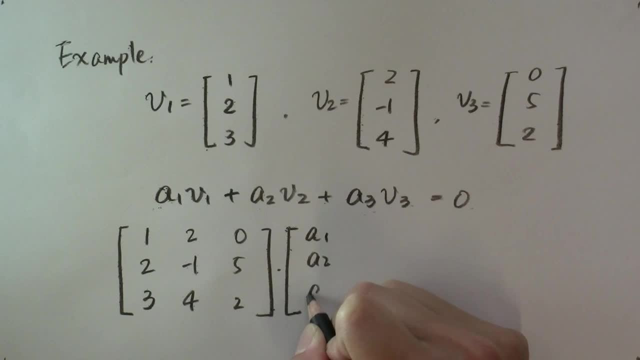 vector, a sub 1, a sub 2, a sub 3 equal to 0.. What I just did is listing all these column vectors as the three columns of a matrix, because this expression is exactly equal to the matrix vector multiplication here, And we recognize that this is a linear system. What kind of a linear system? 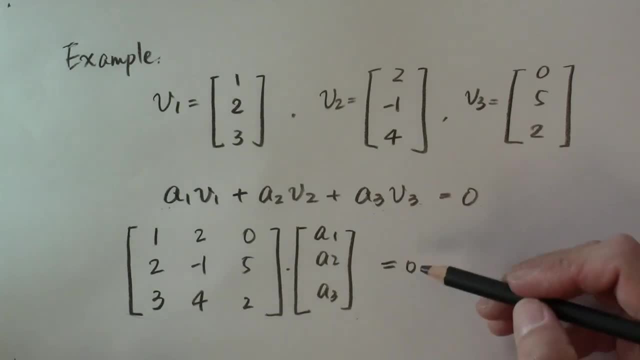 is this? That's right, it is a homogeneous system because the right-hand side is the zero vector And we recognize that this is a linear system. What kind of a linear system is this? That's right, it is a linear system because the right-hand side is the zero vector. If I write it: 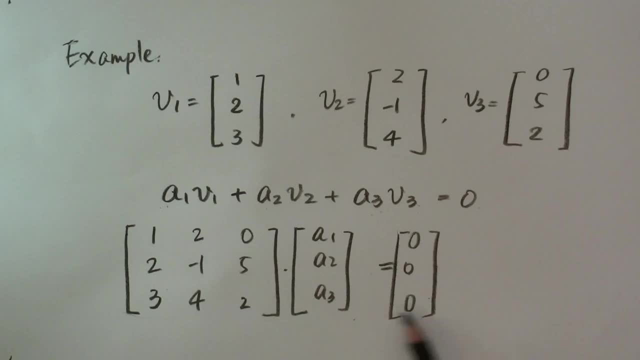 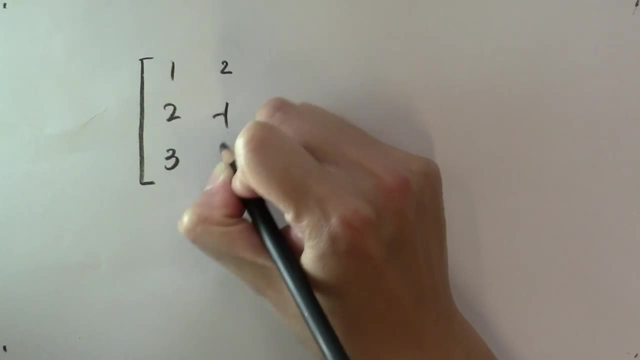 out. it's actually this zero vector. And how do we solve this system? Again, we form the auxiliary matrix 1, 2, 3, 2, negative. 1, 4, 0, 5, 2, 0, 0, 0. And use row reduction to reduce that to echelon. 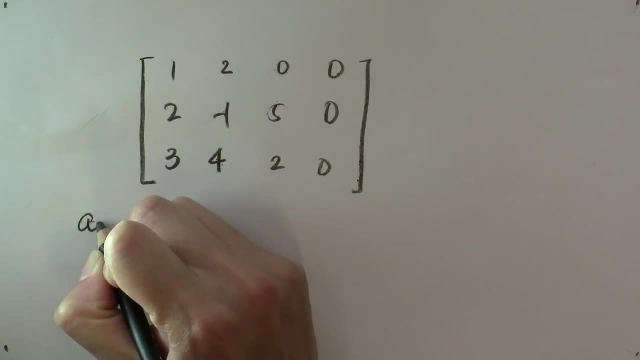 form And in the end, we find the solution to be: a sub 1 is equal to negative. 2, a sub 3, a sub 2 is equal to a sub 3, a sub 4, a sub 5, a sub 6, a sub 7, a sub 8, a sub 9, a sub 10, a sub 11,, a sub 12, a. 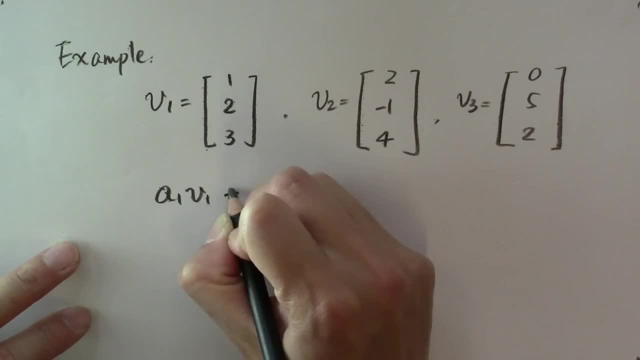 look at the equation: a sub 1 times v- sub 1 plus a sub 2 times v- sub 2 plus a sub 3 times v- sub 3, equal to the zero vector. If there is a set of numbers- a sub 1, a sub 2, a sub. 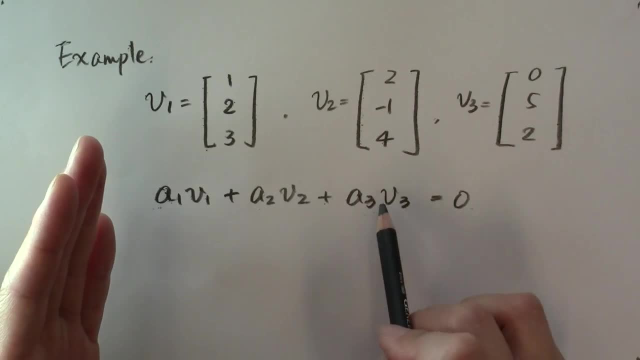 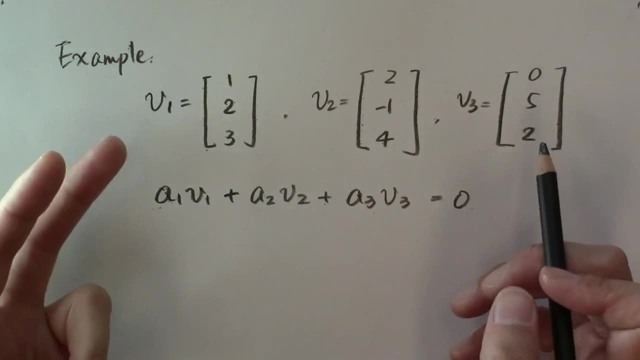 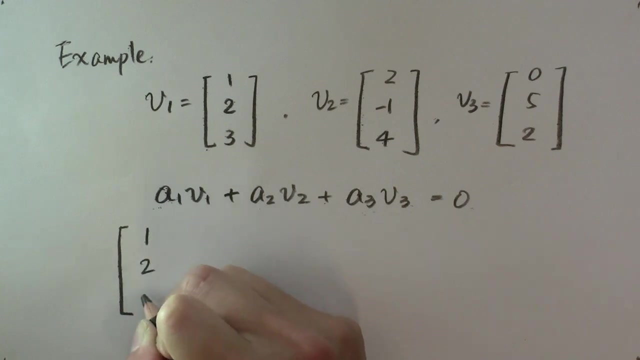 3 that satisfy this equation and they're not all zeros, then this set of vectors is not linearly independent. Otherwise it will be linearly independent And we recognize that the left-hand side is exactly the equation: 1, 2, 3, 2, negative, 1, 4, 0, 5, 2, 3, 4,. 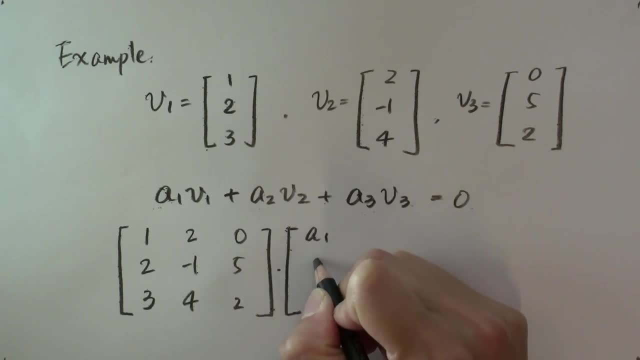 multiplying the vector, a sub 1, a sub 2, a sub 3 equal to 0.. What I just did is listing all these column vectors as the three columns of a matrix, because this expression is exactly equal to the matrix vector multiplication here And we recognize that this is a linear. 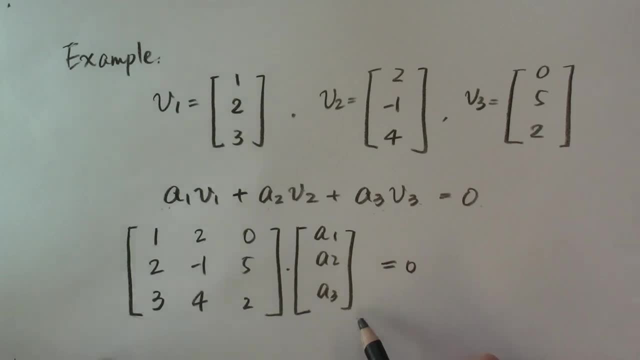 system. What kind of a linear system is this? That's right, it is a homogeneous system because the right-hand side is a linear system, The left-hand side is the zero vector. If I write it out, it's actually this zero vector. 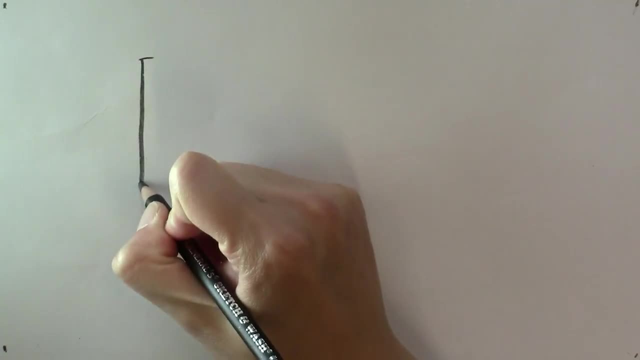 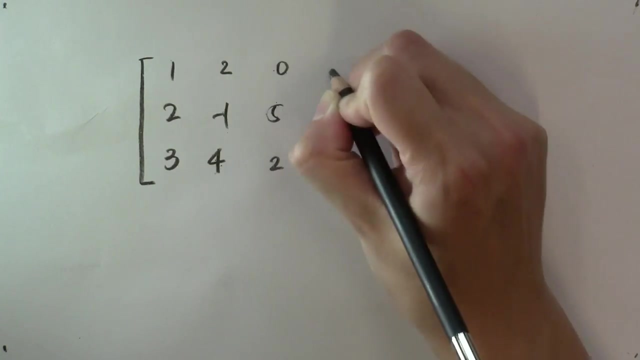 And how do we solve this system? Again, we form the auxiliary matrix 1, 2,, 3, 2, negative 1, 4, 0, 5, 2, 0, 0, 0. And use row reduction to reduce that to echelon form And in the 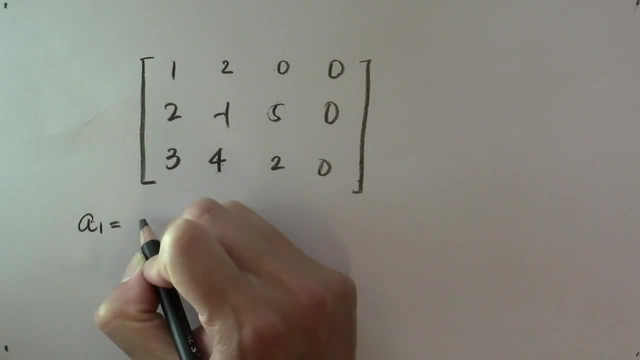 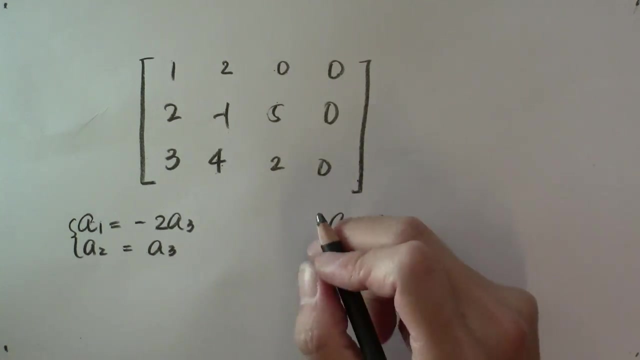 end we find the solution to be: a sub 1 is equal to negative. 2, a sub 3, a sub 2, a sub 3.. We're going to set a sub 3 to be anything. Let's say a sub 3 is equal to 1.. Then that 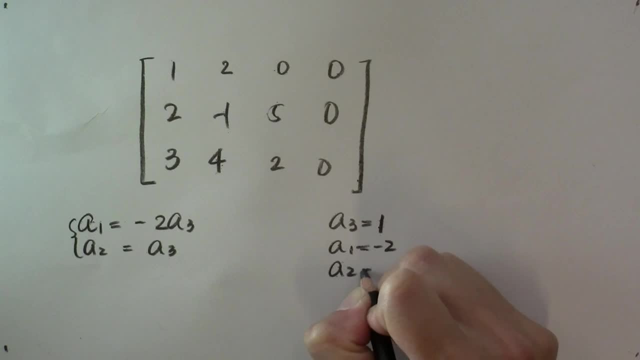 means a sub 1 is negative, 2.. a sub 2 is 1. And that is a set of coefficients satisfying this equation. So if we write it out, negative 2v sub 1 plus v sub 2 plus v sub 3 is equal. 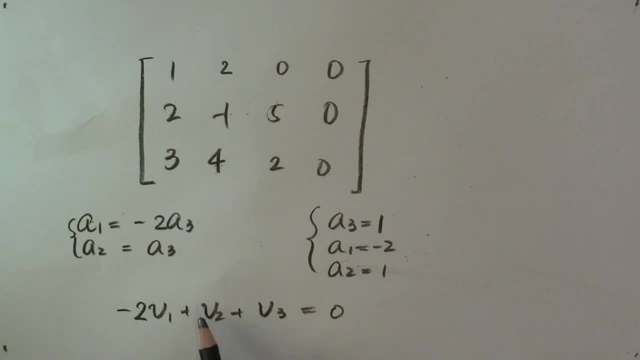 to the zero vector. So what we're going to do is write it out And since we found a set of coefficients, we're going to write it out, And that's a set of coefficients satisfying this equation, coefficients that are not all 0 satisfying this equation. then, by definition, the vectors: